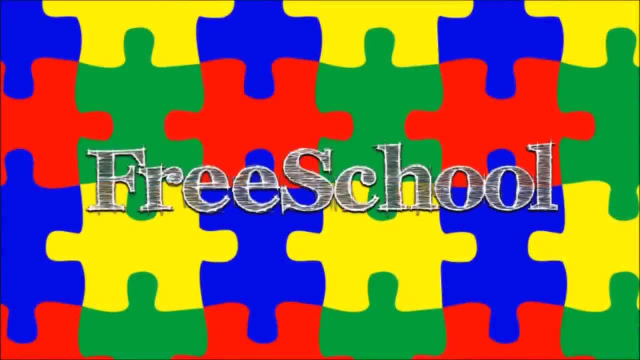 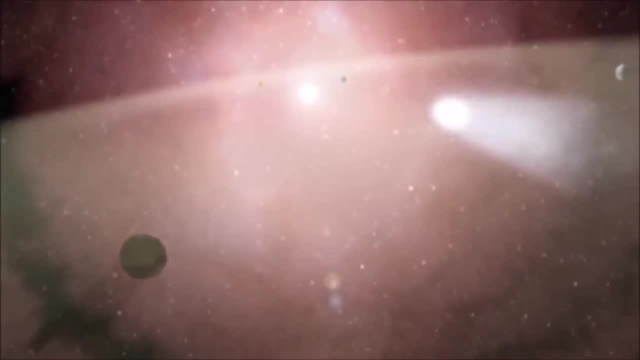 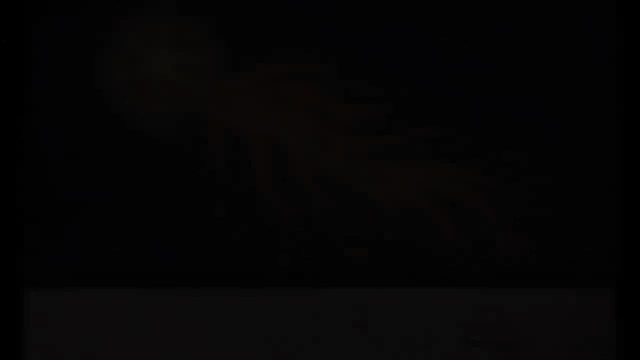 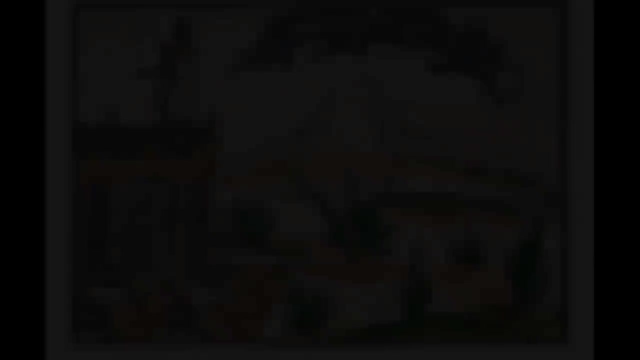 You're watching FreeSchool. Born in the dark outer reaches of our solar system, comets are lonely wanderers. For thousands of years, comets have drawn the attention of philosophers and astronomers. Many ancient peoples from cultures all over the world believed that comets were a sign. 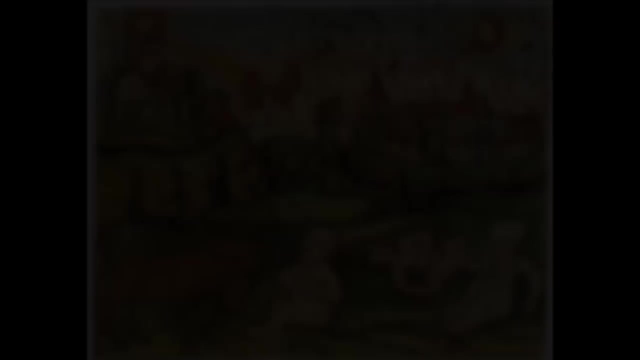 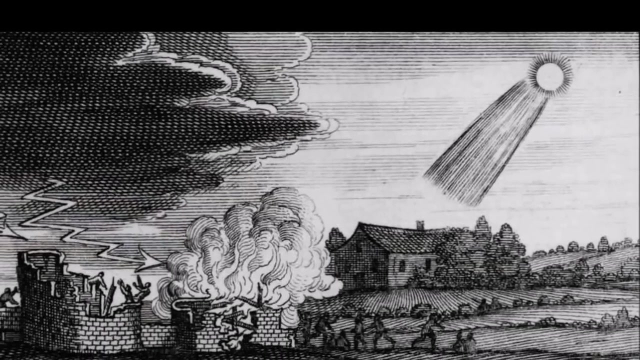 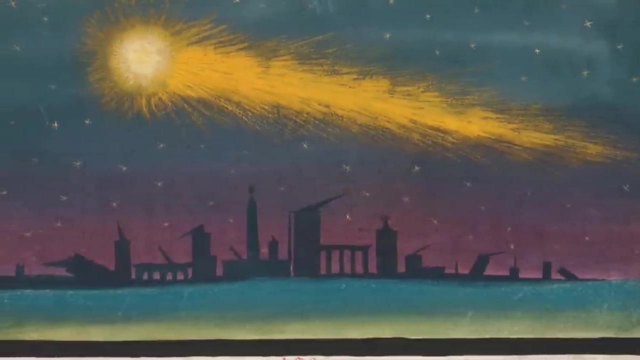 either of good fortune or disaster. Comets were thought to be fireballs or hairy stars traveling through the upper atmosphere. That is where they got their name. The word comet comes from a Greek word meaning wearing long hair, referring to their long, bright tails. 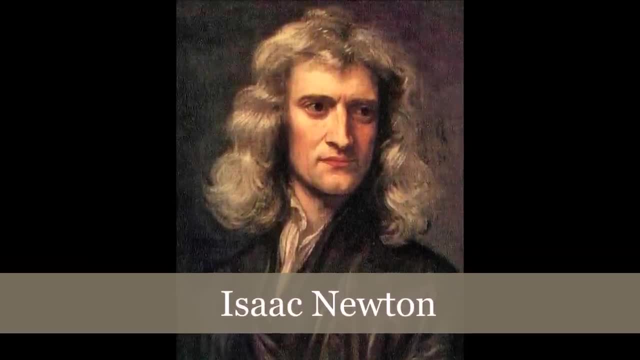 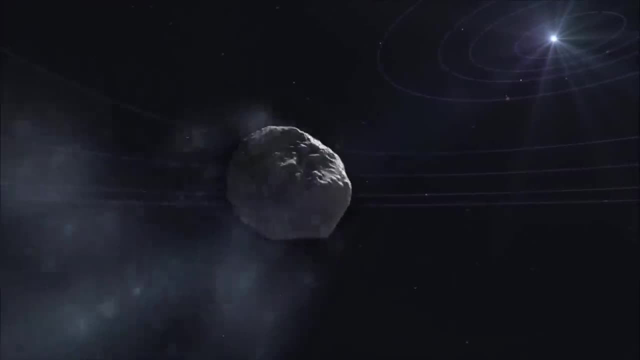 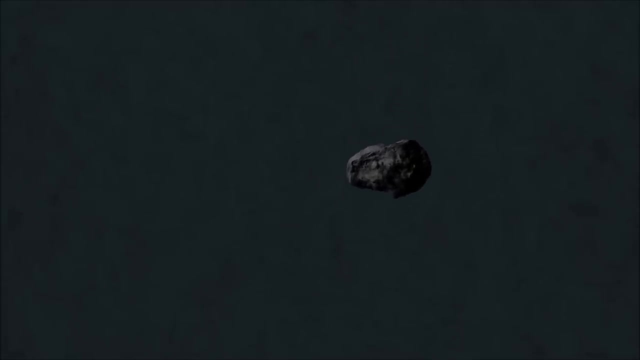 It was Isaac Newton who described comets as solid bodies with thin tails of vapor heated by the sun, A description supported by modern astronomical observations. Comets are similar to asteroids, But unlike asteroids, which are mostly rock and metal with small amounts of ice. 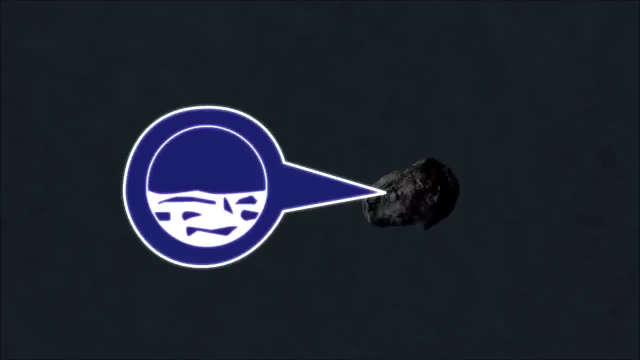 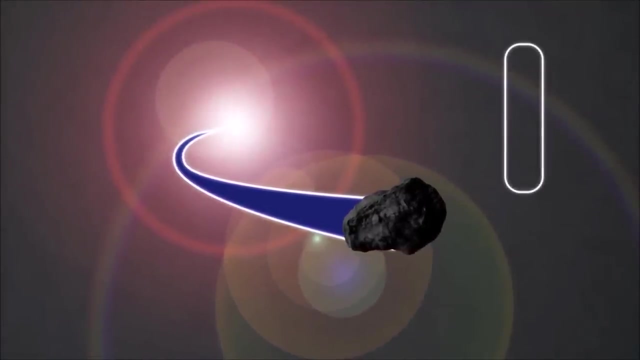 comets are made of ice, dust and frozen gases. Because of this, comets are often called dirty snowballs. While out in deep space, they are unremarkable lumps of ice and rock, But as they enter the inner solar system and come closer to the sun, they begin to heat up. 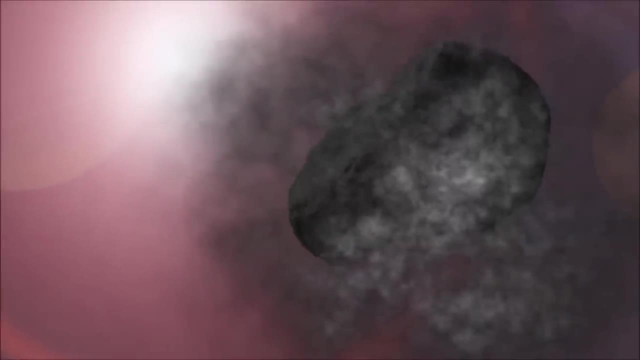 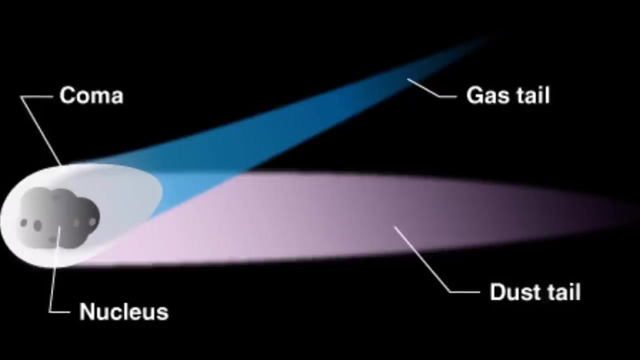 The comet's ice begins to sublimate or turn directly into gas. This gas creates a cloud around the comet, making it seem fuzzy. There are three main parts of a comet: The nucleus, or solid central structure made of rock, dust and ice. 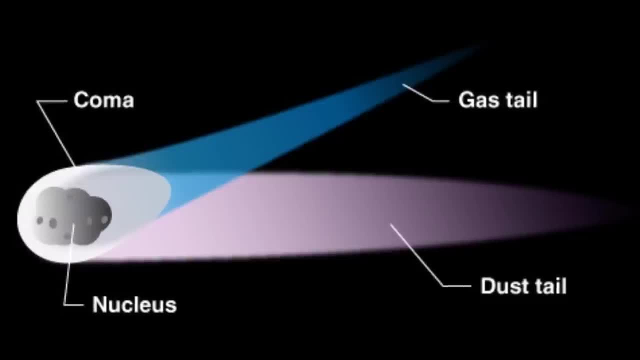 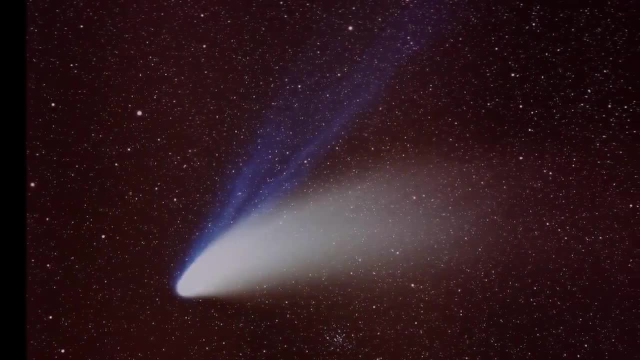 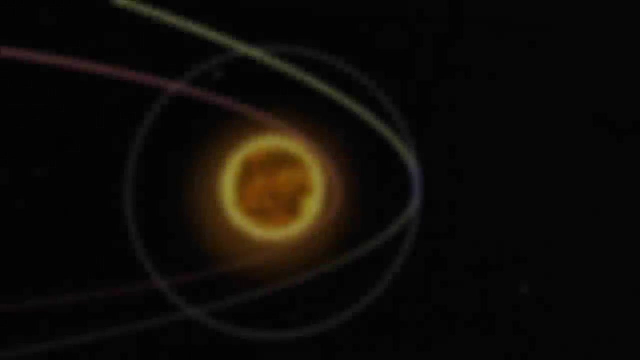 The coma, or dust and gas forming a thin atmosphere around the nucleus And the tails. Comets generally have two different tails. One is made of gases, the other is made of dust. These two tails usually point in different directions. The gas tail is blown directly away from the sun by the solar wind. 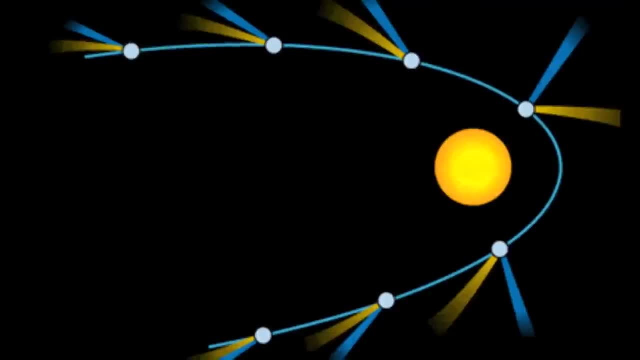 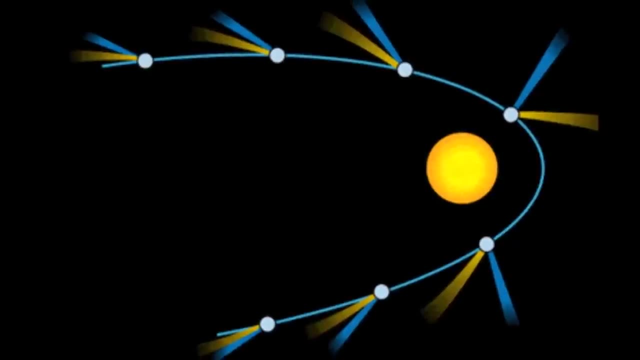 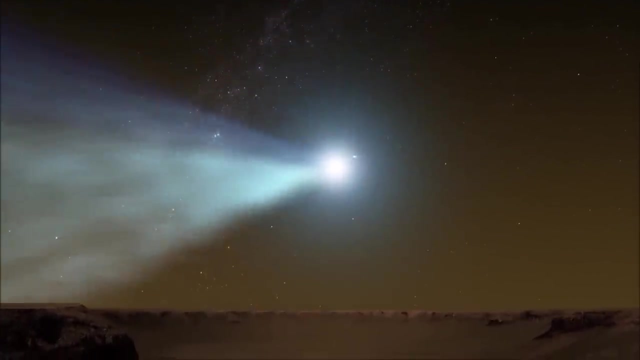 No matter which way the comet is traveling, this gas tail will be pointing away from the sun. The second tail is made of the dust released by the comet. The dust tail usually points back along the comet's path. A comet's tail may stretch as far as 6 million miles or 10 million kilometers long. 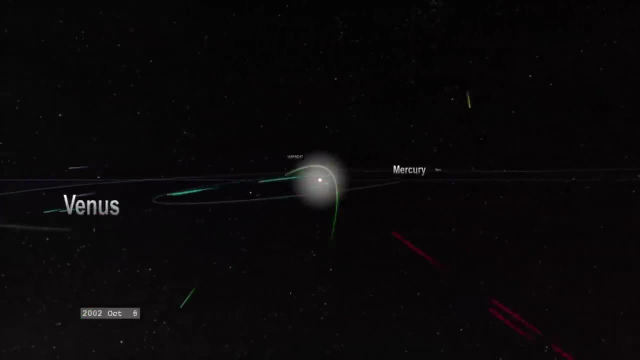 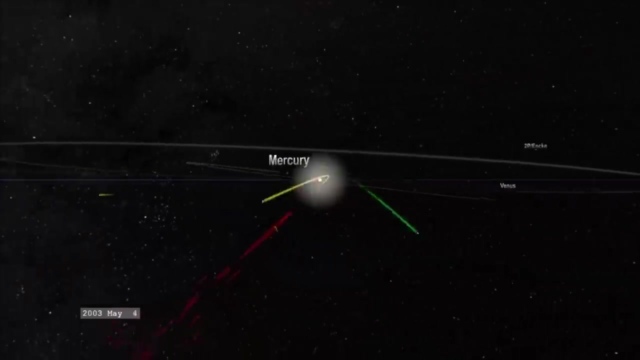 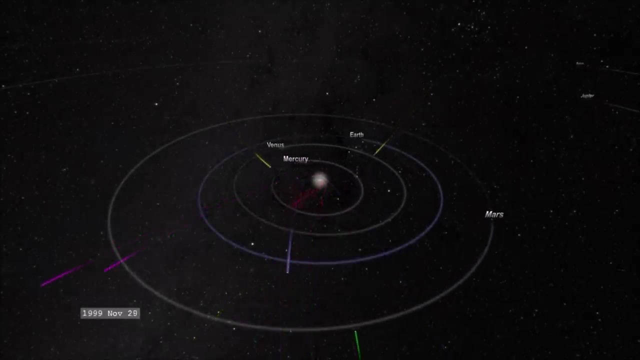 The orbit of a comet is usually elliptical or oval in shape and may have a length of only a few years or as many as millions of years. Comets may be classified by the length of their orbits. Periodic or short-period comets are comets that orbit the sun in less than 200 years. 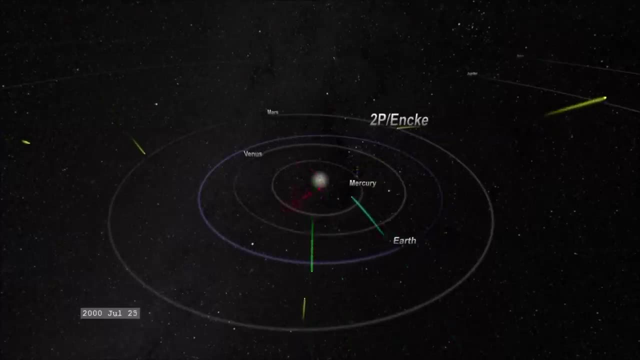 Comets with orbits of 200 years to 1,000 years in length are called long-term comets, And comets that take more than 1,000 years to orbit the sun are called near-parabolic comets. Some comets, called hyperbolic comets, pass by only once and then exit the sun. 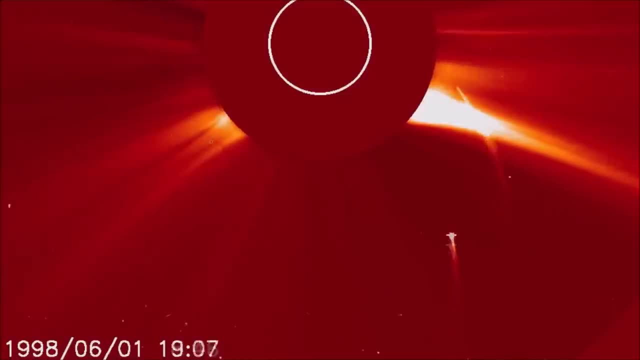 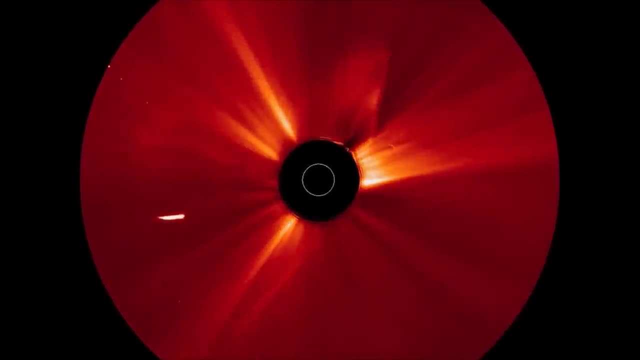 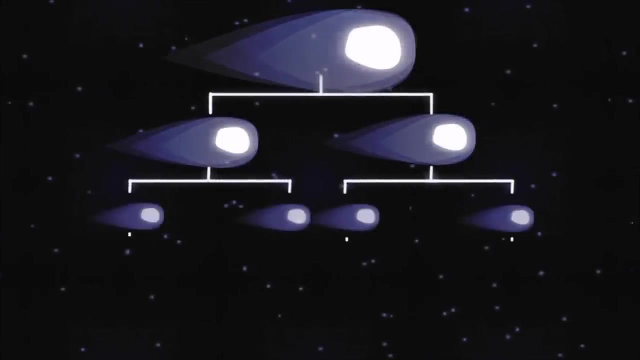 Comets that pass extremely close to the sun are called sungrazing comets. Some large sungrazers survive to go around the sun over and over again. Other comets travel so close to the sun that they evaporate or break into fragments and are destroyed. 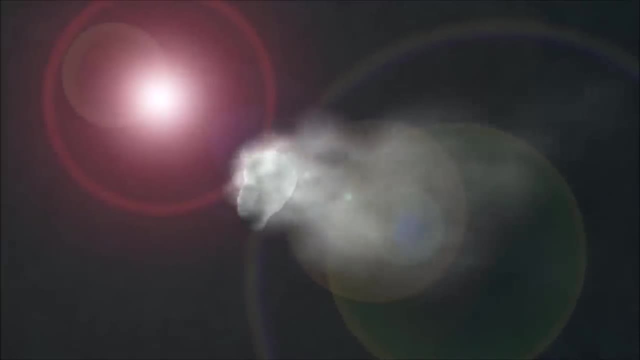 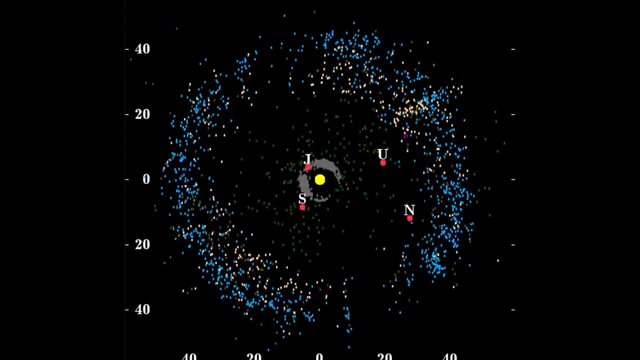 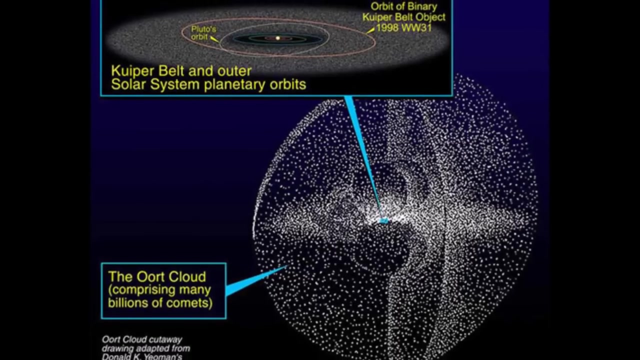 Comets are believed to come from two places on the outskirts of the solar system: The Kuiper Belt, a region past Neptune filled with asteroids, dwarf planets, comets and more, and the Oort Cloud, a sphere of icy leftovers from the creation of the solar system nearly a light-year away from the sun. 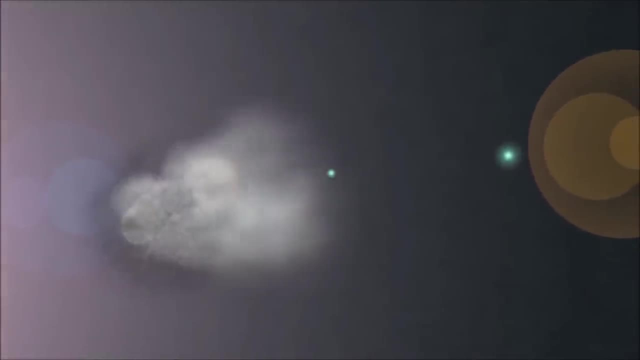 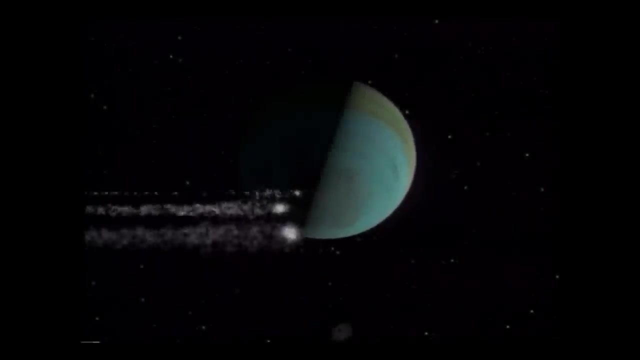 Scientists believe that short-period comets come from the Kuiper Belt and long-period comets come from the Oort Cloud. Because these comets are made of ancient material and come from so far away, astronomers love to study them as they come near. 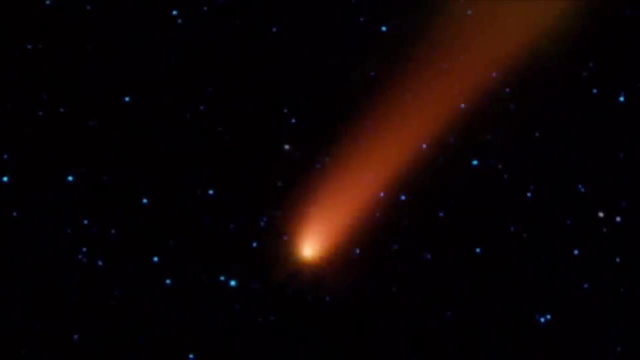 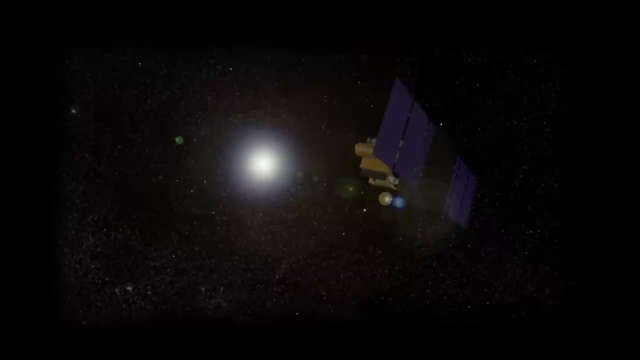 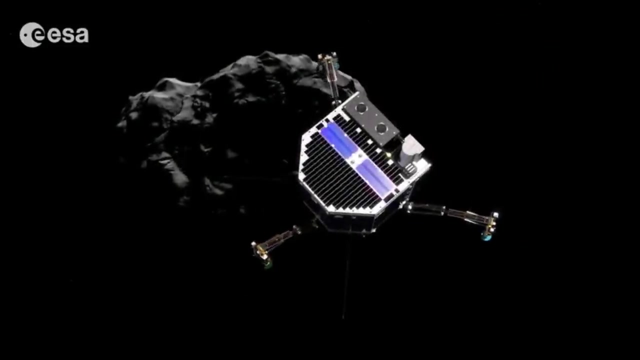 In the past, comets could only be studied through ground-based telescopes, but over the last 30 years, spacecraft and probes have been used to visit and observe comets. In 2014,, the European Space Agency's Rosetta space probe successfully landed on the surface of a comet.